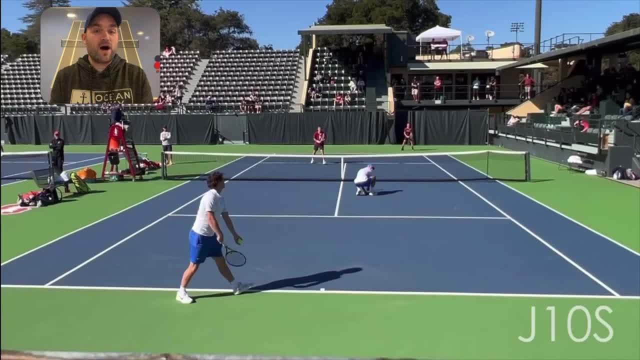 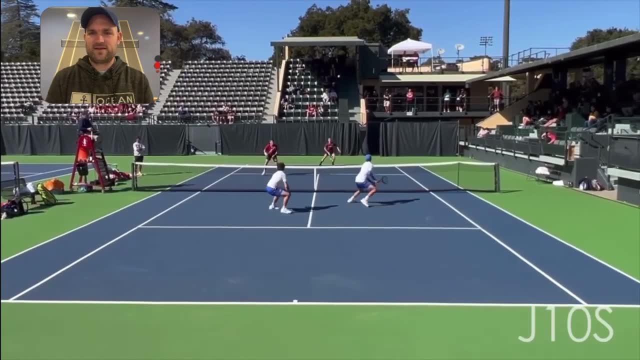 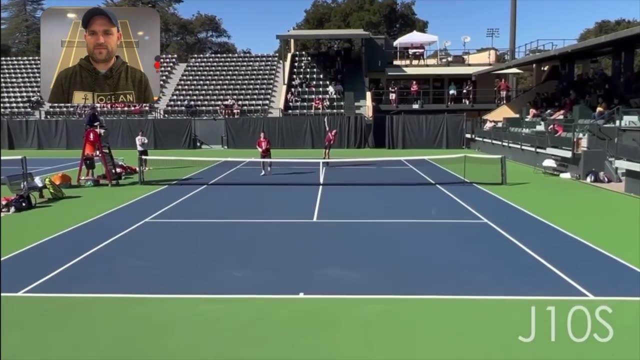 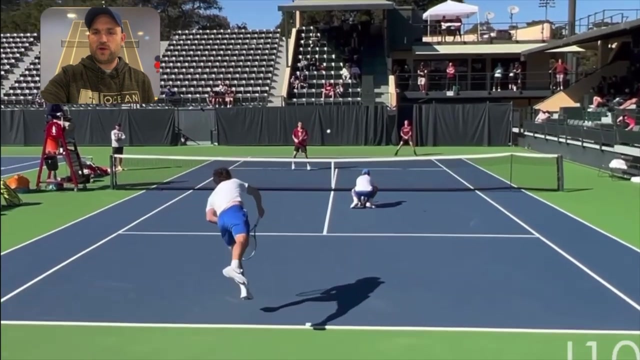 awesome channel. I've put their link in the description below, So let's watch this short point and then we'll analyze it. All right, so right off the bat, we can see the servers are in an eye formation. So in this, 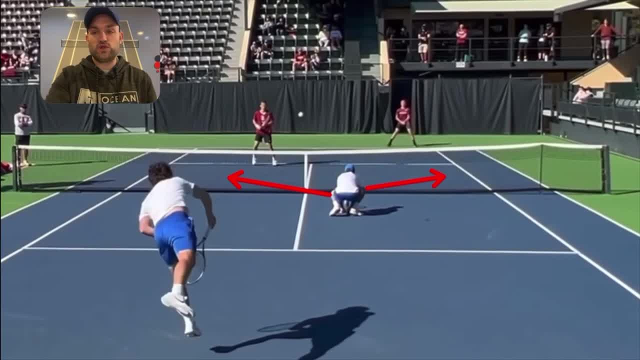 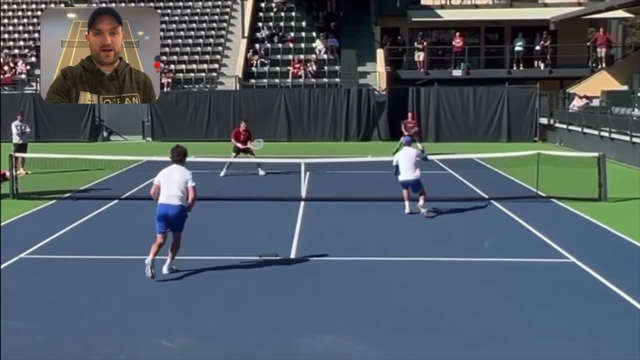 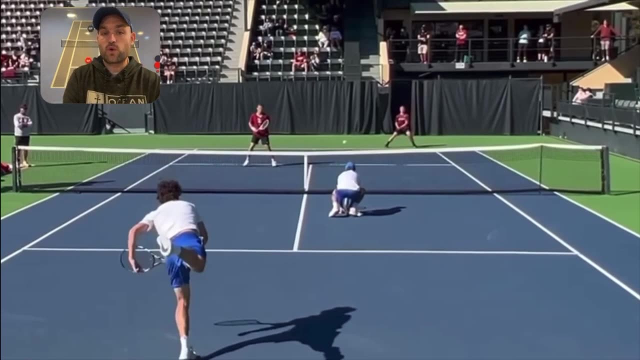 scenario: the net player is either going to move to his left or to his right. Now, it's really smart that the net player moves to his right in this scenario. Here's why, When you serve in doubles, you can either serve to the inside ground stroke or to the outside ground stroke. 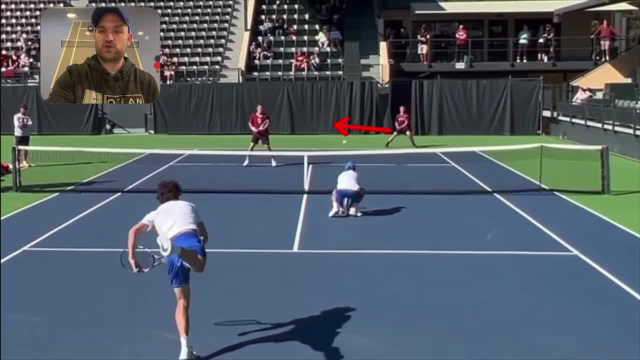 The inside ground stroke is on the side, toward the center of the court. The outside ground stroke is toward the outside of the court. So inside ground stroke, outside ground stroke. It just so happens that the inside ground stroke gets ripped up the line very often and the outside ground stroke gets pulled. 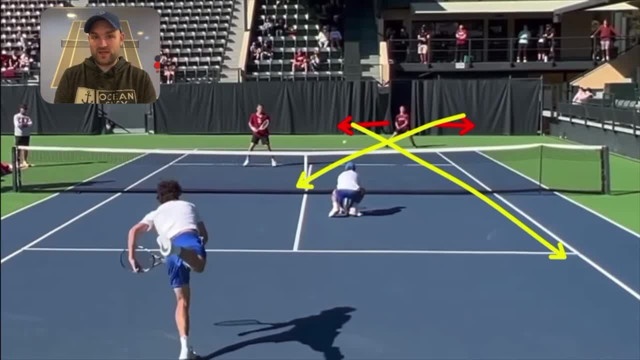 cross court. very often It's a bit counterintuitive, but when you serve down the tee in doubles- and maybe not the tee but definitely right to the inside ground stroke- that ball gets pulled down the line over and over again. So you can see, the serve goes to the inside ground stroke and the 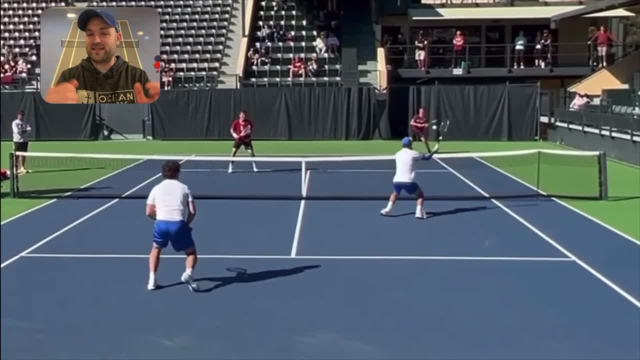 server covers the alley. This is definitely premeditated. The server and the server's partner are on the same page. It was super smart for them both To do what they did. Now, if the serve had gone out wide, you would want the net player to have. 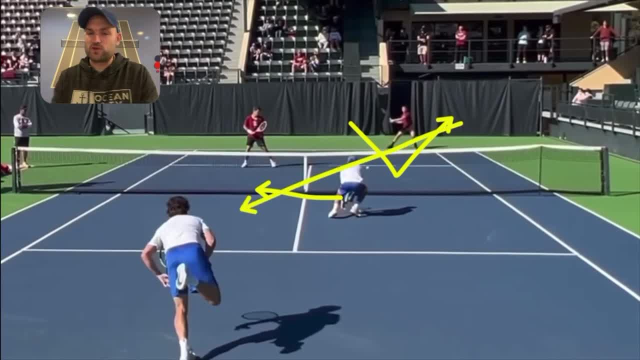 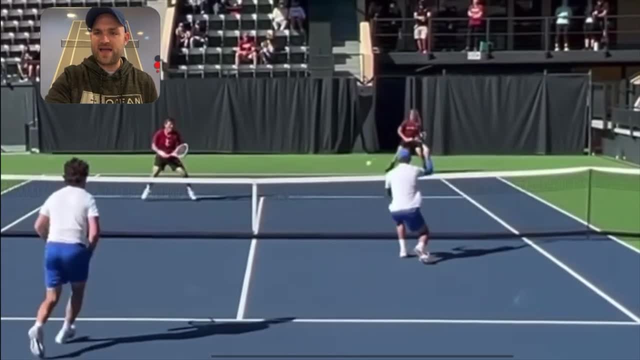 moved cross court because that backhand, especially for a right-hander, is most likely going to get pulled cross court. So now let's check out the net player. when he pops up. He pops up, he gets a high volley. He doesn't do much with the volley. Let me show you why: Watch when he pops up. When he pops. 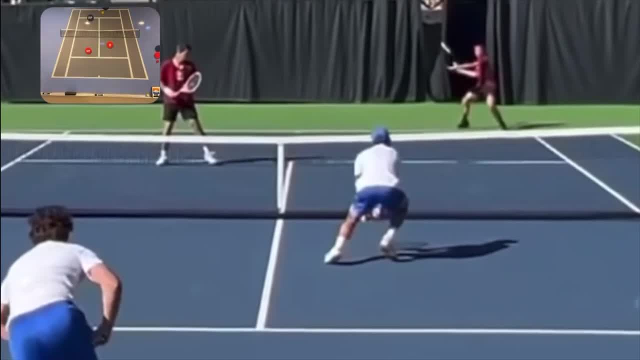 up. he drags the racket and keeps it low. Let me actually get a racket here. Watch what he does. He's down here and his racket is low And when he pops up, his racket's still down When you pop up. 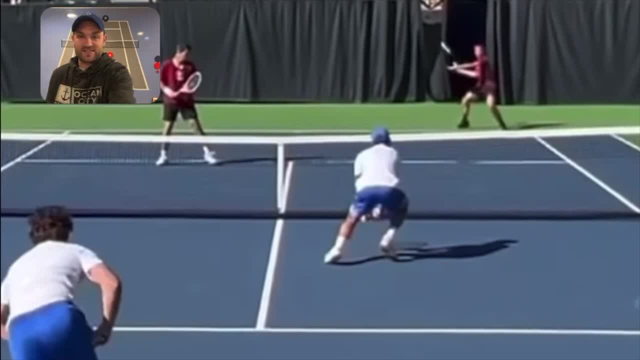 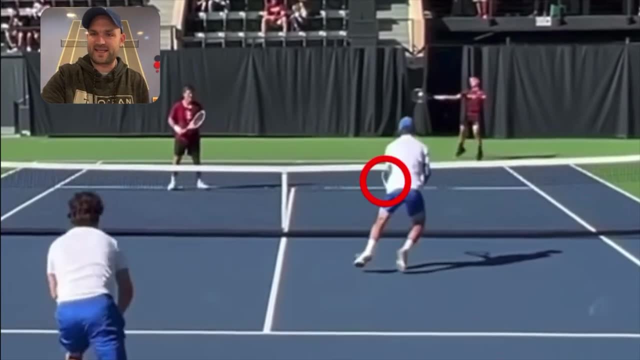 you want your racket up Because his racket isn't up. he's actually late with his racket. He doesn't quite do much with it, Like right there you can see he's fully popped up, but the racket's still down below net level, And so it makes him late on a ball that's coming right above his head. 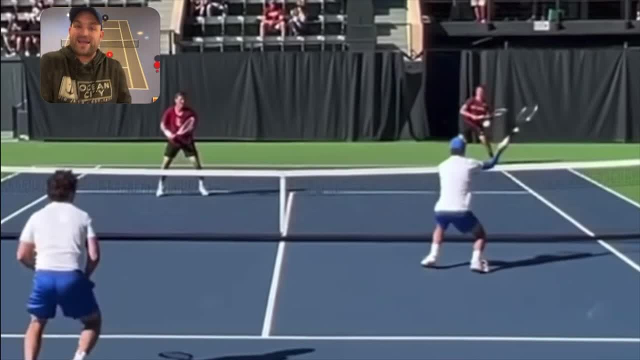 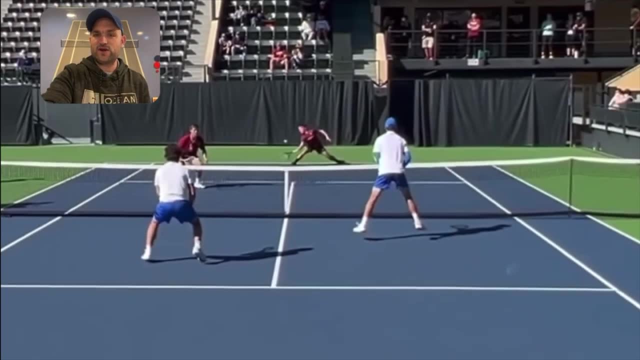 So you want that racket up, especially when you pop up. don't pop up with your racket still down below net level. So he doesn't do much with this volley. He tries to split the uprights hitting between them, And then here a lob occurs right over their 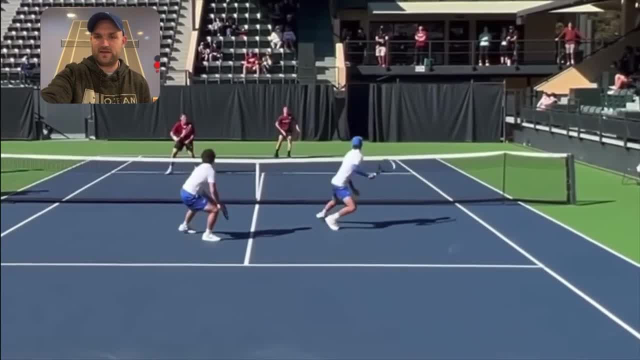 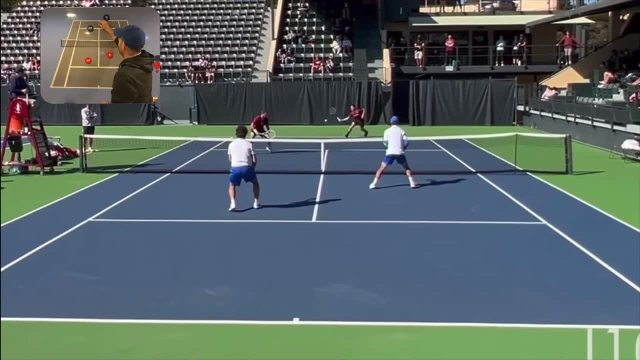 heads and they have to run back. So let's talk about what just happened right there, or what should happen and what happened. So let's create this scenario on the strategy board: So here's the returner with a ball in the middle and he hit a lob down the line. If this is you. 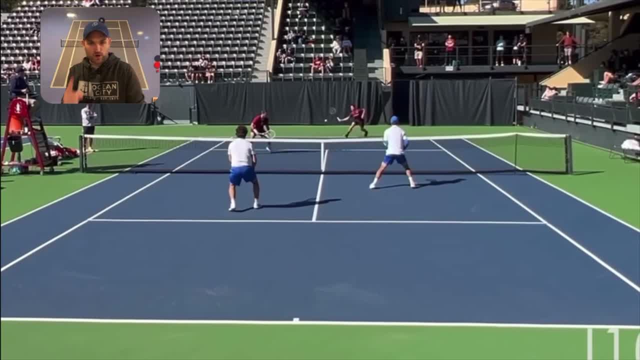 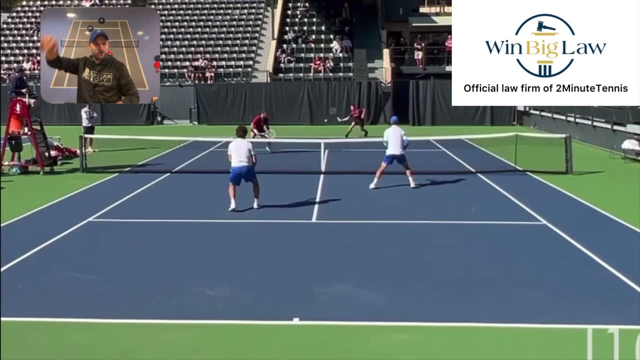 and a ball goes over your head. your number one priority is to see if you can hit an overhead. right, You're trying to go back and see if you can hit the best shot possible, Which would be kind of a scissor kick overhead while moving backward. So while you're busy, 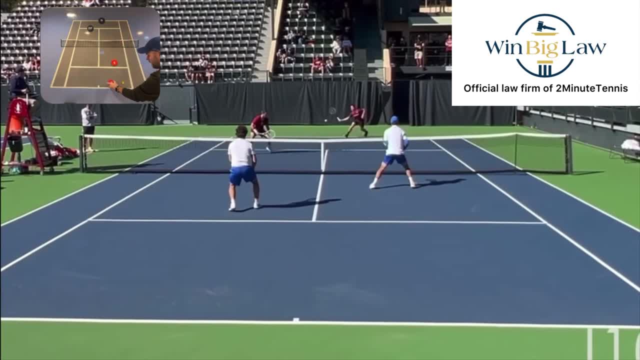 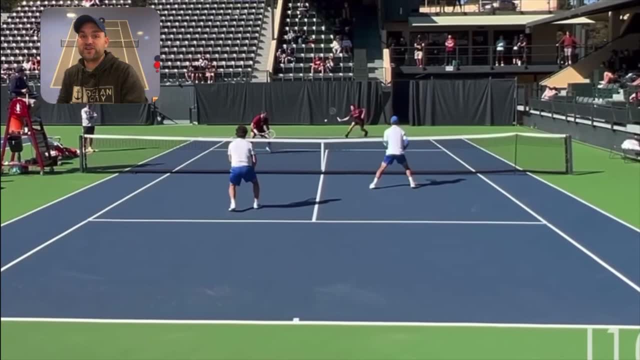 moving back. your partner should be doing their job to come back in case you can't get that lob that's going over your head. See when the ball goes over your head and doubles. you're either going to say mine or you're going to say yours, and you're going to have to switch This player. 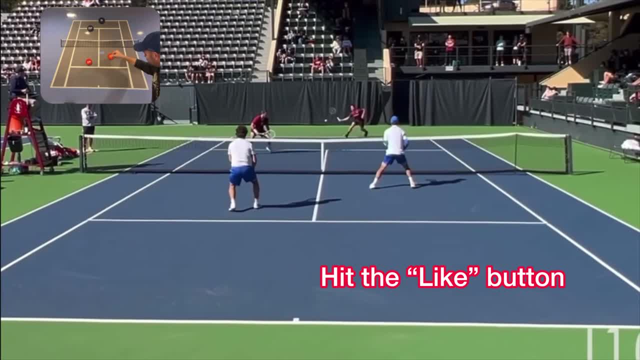 shouldn't wait to hear what happens When the ball goes over your head as you're going back. they don't care what you say, They're running back right away. If you say you've got it to slam an overhead, then they go back, But if you say yours, please switch this partner. the partner should have. 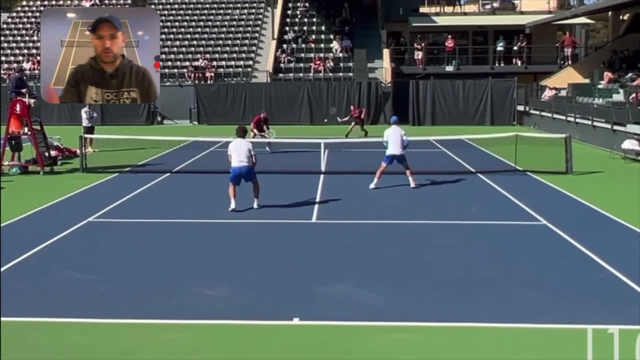 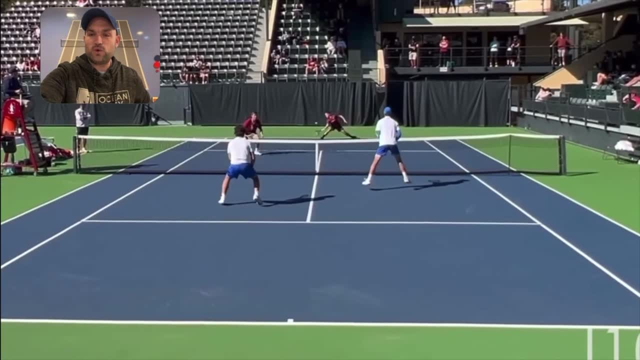 already gone back to get it and this player or you then switch. Watch what happens. The net player here, he doesn't go anywhere when the lob occurs, He just holds his ground, He moves a little bit and the guy who's being lobbed looks and says: hey, buddy, go get it. He's like 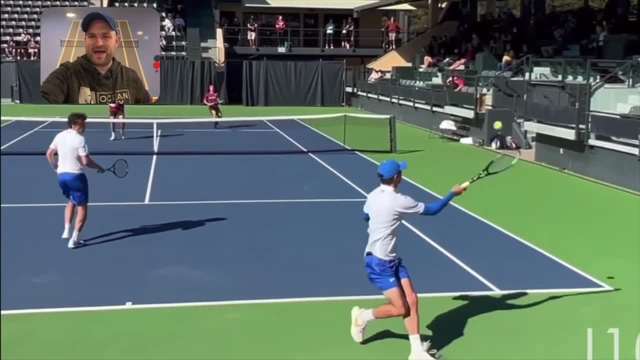 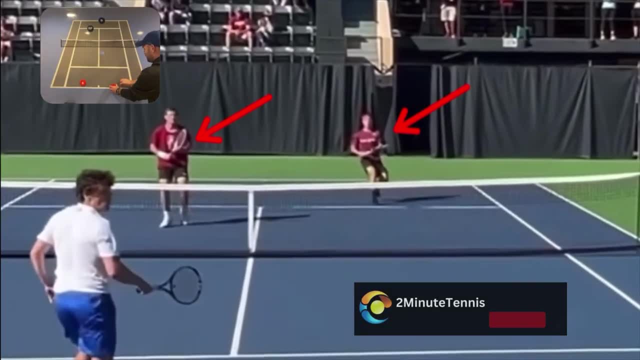 wait a minute. my partner didn't go get that ball, So now he has to run back. Now a couple of things. Let's look at these guys. Where should they be going When you lob your opponent successfully? so let's say you're the blue team. now When you lob successfully over, 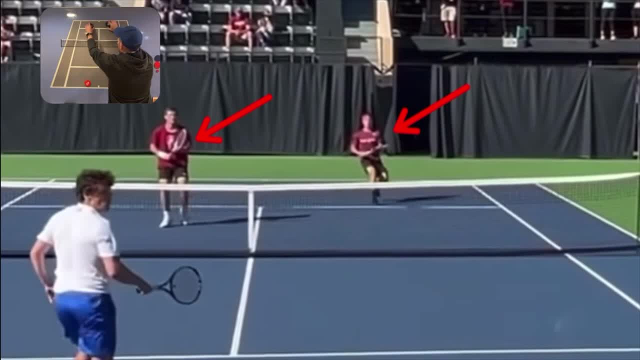 your opponent's heads and let's say they switch, you and your partner should put your toes on the service line. Write this in stone, Etch this in your mind When you lob your opponents: put your toes on the service line. Whether that means you move back or move forward, it doesn't matter You. 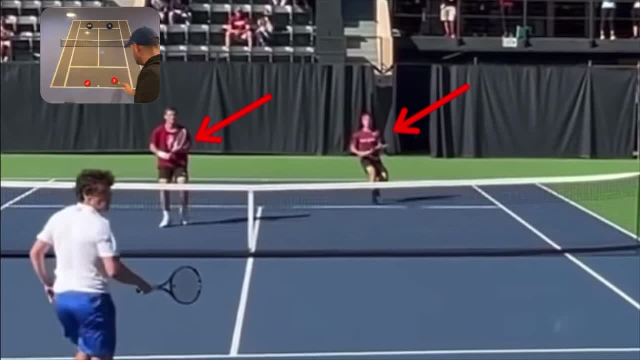 need to put your toes on the service line When you lob your opponents. put your toes on the service line because you're expecting a lob back And if your toes are on the service line, if it's a great lob and nice and deep, you can go back. If it's a bad lob, you can come forward If it comes right. 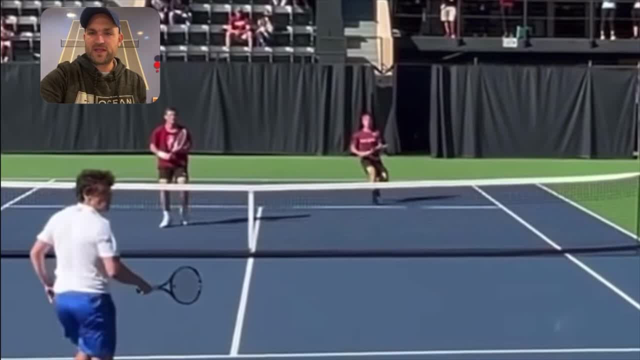 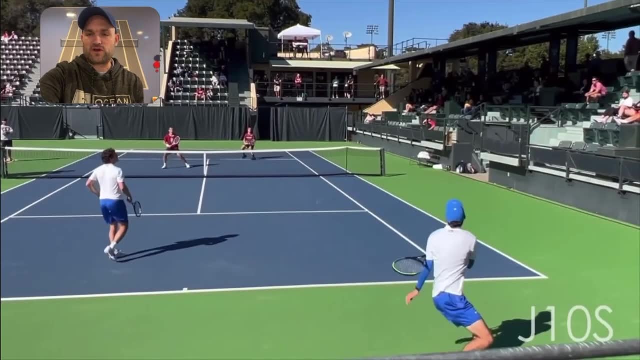 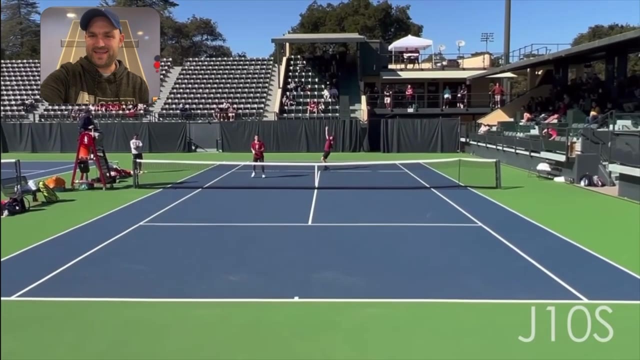 to you. it comes right to you. So watch what happens. This guy gets too close. This guy stops on the service line, which is exactly what you want. So you want to be on the service line. So then a lob goes really high into the air. He lets it bounce and then he misses the overhead All. 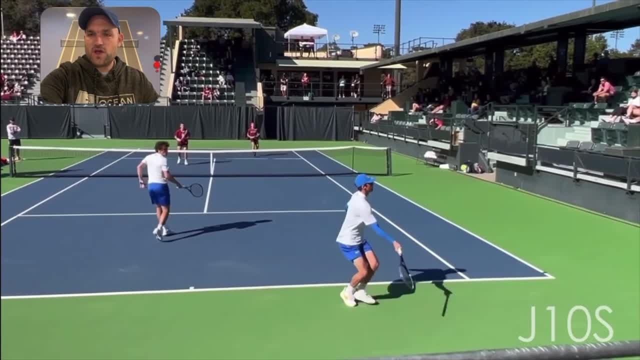 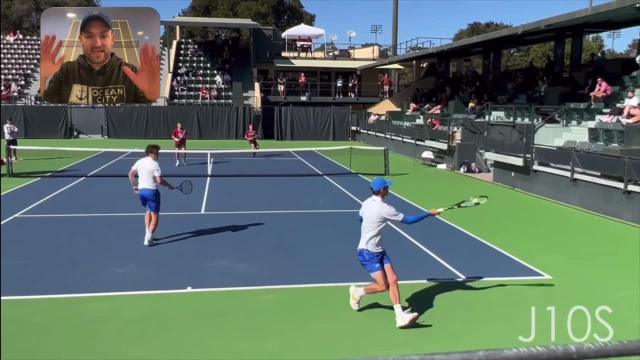 right. So I have a recommendation For you when it comes to hitting lobs. you want to hit lobs especially defensive, when you're running back really high and forget about hitting it deep. Do you know that the number one reason why players miss their lobs long and the ball lands past the baseline? I have people all the 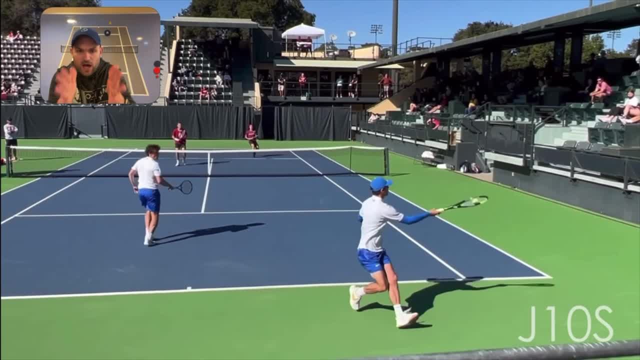 time, Ryan, why do my lobs always land deep Just a couple inches? I just can't get the ball to land in the court. It's because they have the right to land in the court. Ryan, why do you think that the definition of a lob is a ball that goes over your opponent's head? 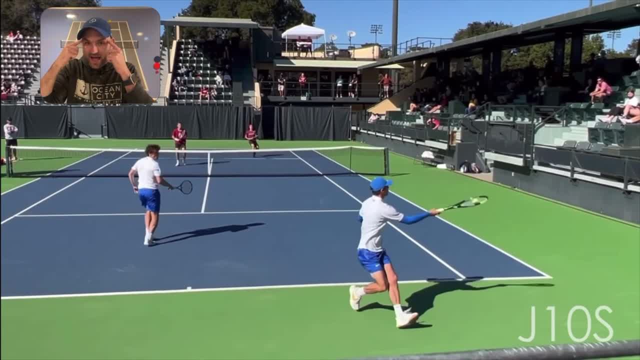 and lands behind them. If in your mind when you lob, you're thinking: I got to get this ball to bounce behind them, Well, no wonder you're missing your lobs long, because if your opponent is around the service line, you're going to try to hit it over their head and get it to land behind them. 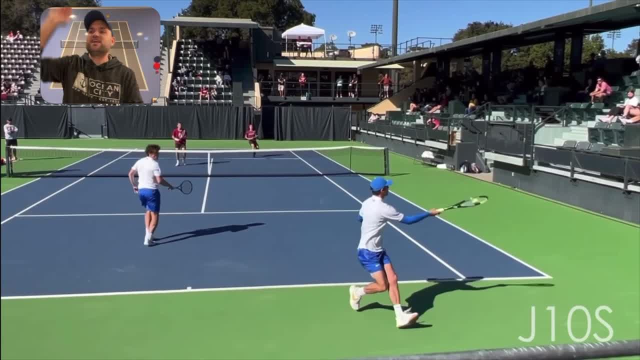 which might have to be three feet past the baseline. Instead of thinking making it land deep, just hit it super high, And I recommend getting the ball up in the air for at least two and a half seconds. So let's see, We got a timer here. Let's see how long his ball. 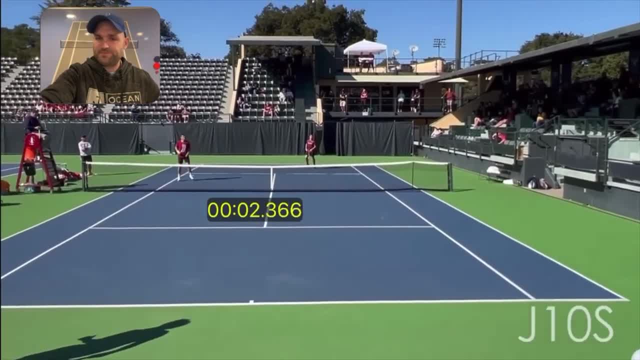 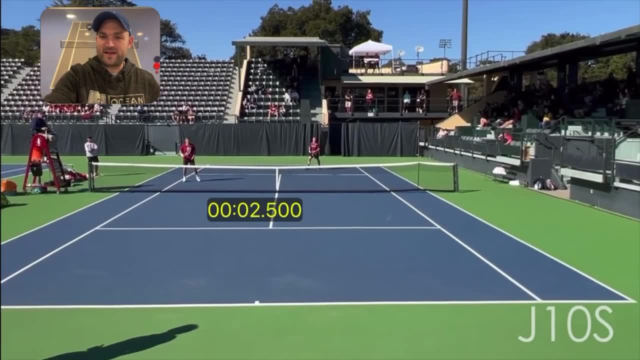 goes up in the air. There's one second. There's- oh goodness, goodness, goodness, I already missed it. There's two seconds. There's two and a half. So right there, right. two and a half, So let's. 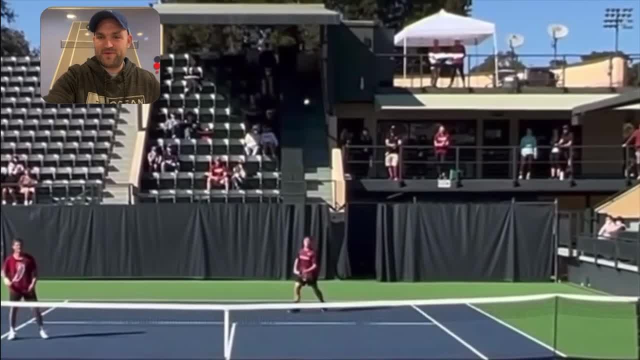 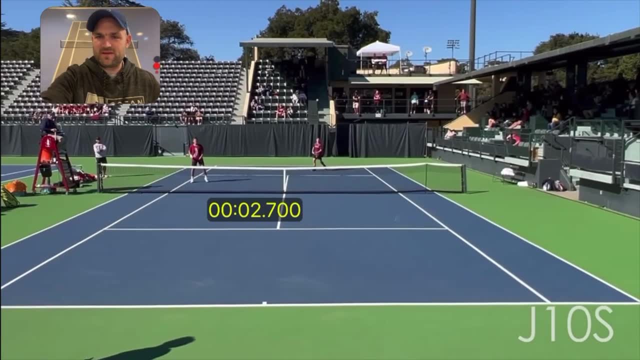 see where the ball is. Man, he got that ball way up in the air. That was amazing. So already 2.6, so the ball is bouncing. Oops, I didn't mean to get rid of put that timer down. Sorry, it's my. 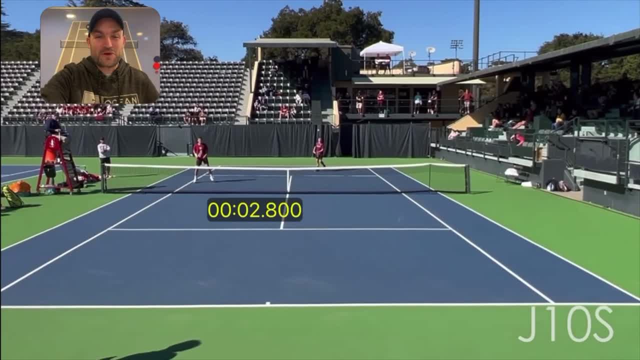 first time using this app, So you're watching it live as I struggle my way through this app. It's called OnForm, by the way. I'll put it up on the screen: OnForm. it's a great app, So check this. 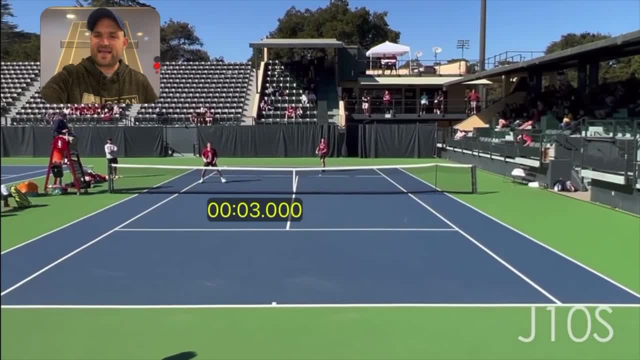 out. The ball bounces right around three seconds, And then what does this guy do? He lets it bounce Now anytime. I suggest that you hit your lob super high in the comment section. I get a lot of viewers and they say, oh man, Ryan, if you did that I would let the ball bounce and then I would. 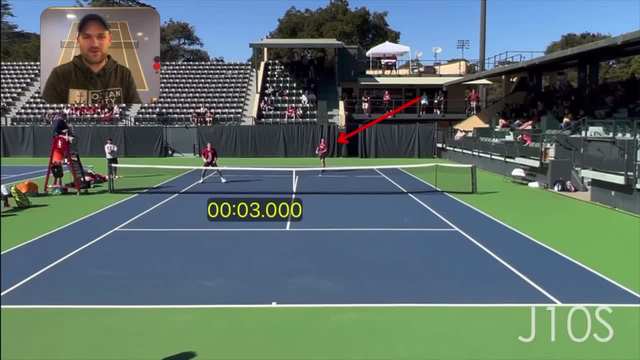 crush it down your throat. I'm like all right. So here's my question to all of you, And I want you to write this in the comment section: When was the last time, with a coach or with a friend, you practiced lobbing super high, letting the ball bounce and hitting it out of the air? I'm 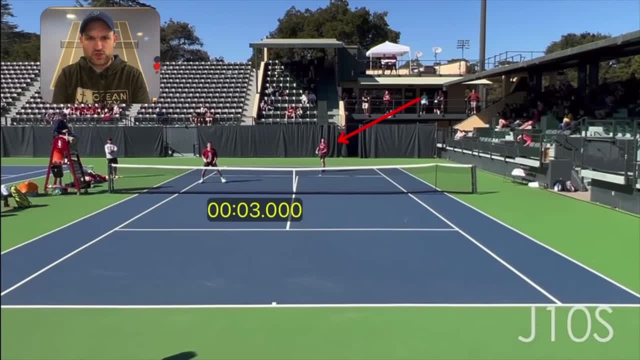 sorry, hitting it off the bounce, hitting it overhead off the bounce. When was the last time you played this fast? Is it for private lessons? semi-private lesson in a team practice? It's really not practiced. So here is a shot that you can force your opponent into hitting and they've 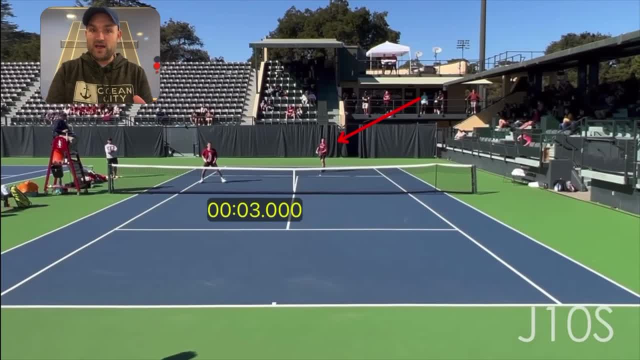 never even practiced it. It is not as easy as the pros on TV make it look, and sure they could hit that ball out of the air, but it is descending so fast as it's dropping nine put meters per second. per second. The chances of them timing that go way down. That's why people let it bounce Here's. 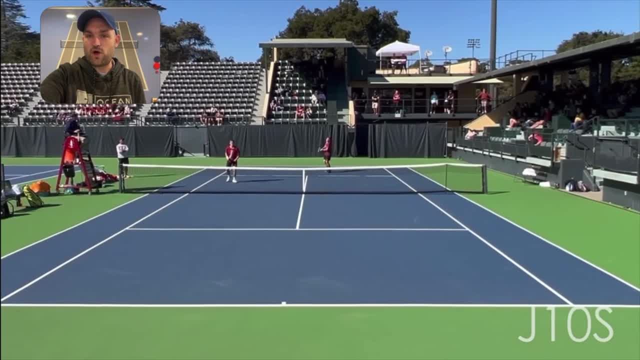 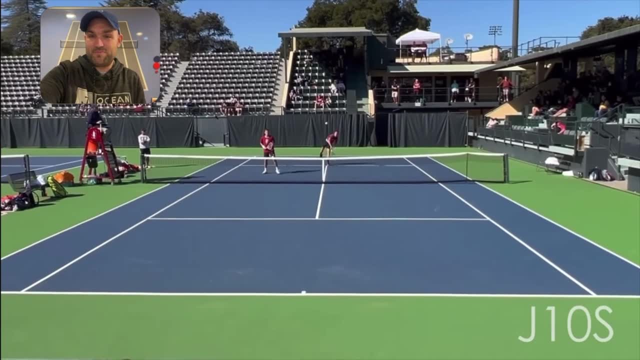 super high level college players and they're letting this ball bounce. So he lets the ball bounce and he hits the overhead and he screws it up, And I would have probably screwed it up too. I can't beat these guys. I don't pretend to be able to beat them. 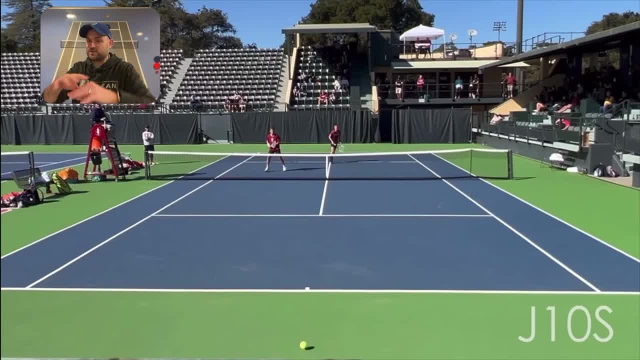 And he hits the ball about two meters long. There was a lot of info there. Film yourself playing and see if you can incorporate some of these ideas. But here's the main idea: When you're running back in doubles or singles, it's the same thing. 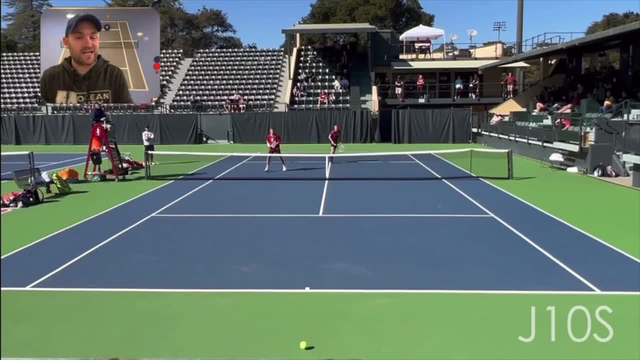 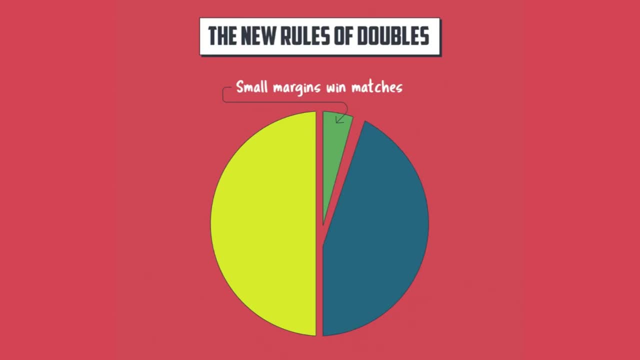 But in doubles- and you're going to lob- hit it super high and the chances of winning go way up. Now, if you need to win more doubles matches, then check out the new Rules of Doubles by Fuzzy Yellow Balls.